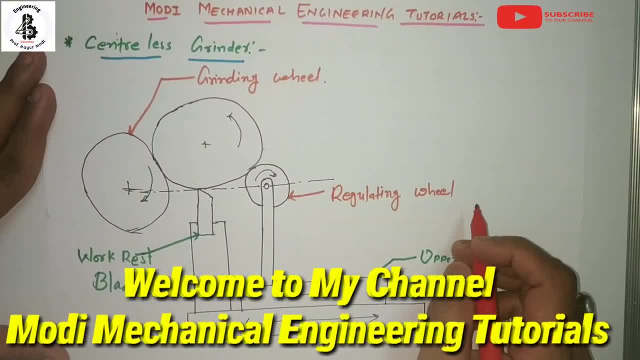 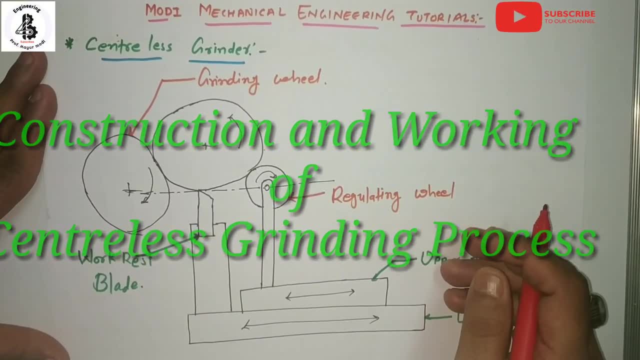 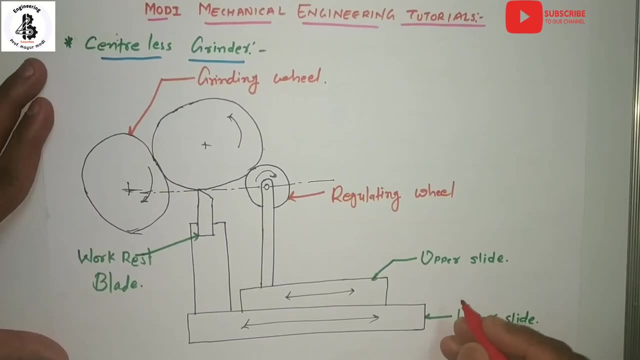 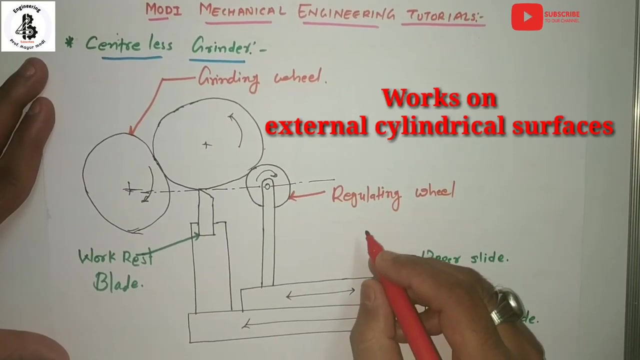 Welcome to my YouTube channel, Modi Mechanical Engineering Tutorials. So today I would like to explain about the construction, working and use of the centerless grinding process. So basically start with the construction of centerless grinder. So basically this will be used for the external cylindrical surfaces, or you can say onto the tapard and form the surface onto the workpiece. 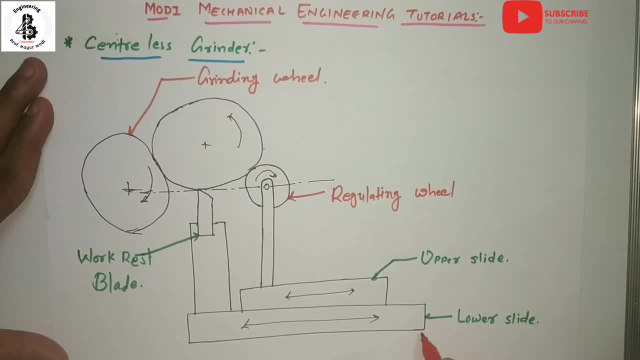 So let us see the basic construction. So that will be the lower side. So that lower side it will be move into the to and fro directions and onto that upper side that will be another sliding moves and on that upper sliding moves that will be attachment of the regulating wheel. So that regulating wheel it will be adjusted according to my shape and size of the job with respect to my workpiece. 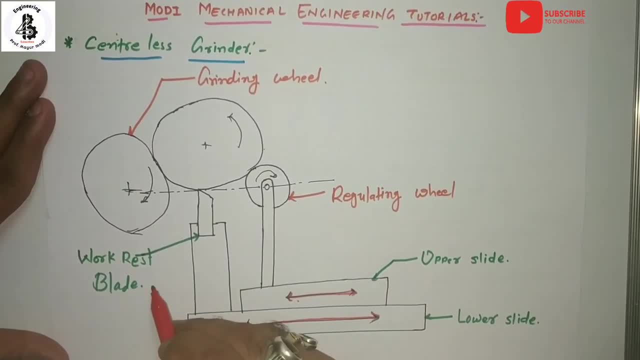 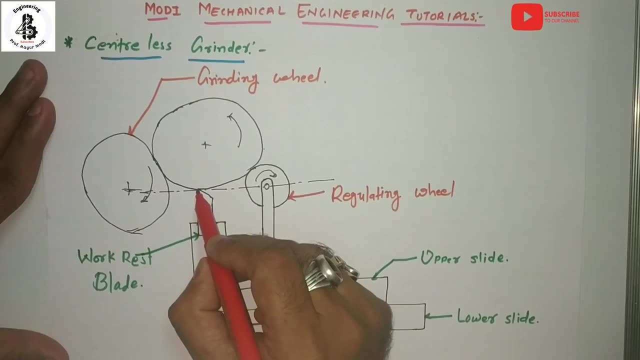 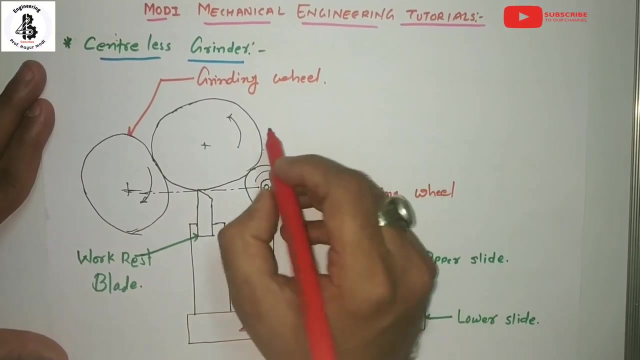 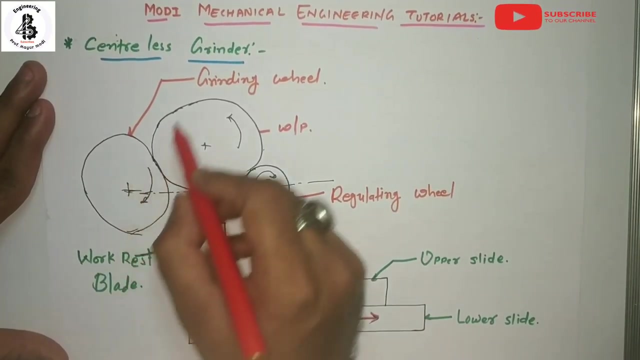 And onto the another side, that will be the work rest blade. So on that particularly work rest blade, our workpiece is being attached and that will be fixed or you can say supported by some another supporting elements. So this one is our workpiece material and for another that will be using of the grinding wheel. 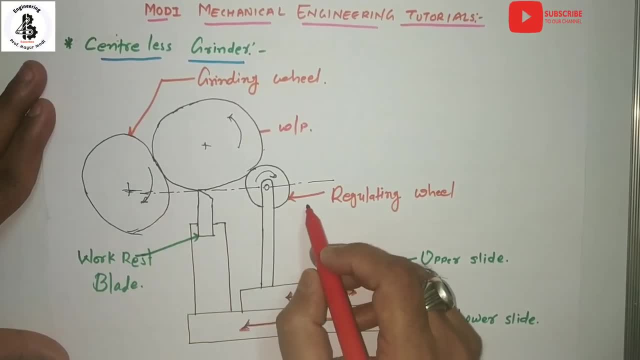 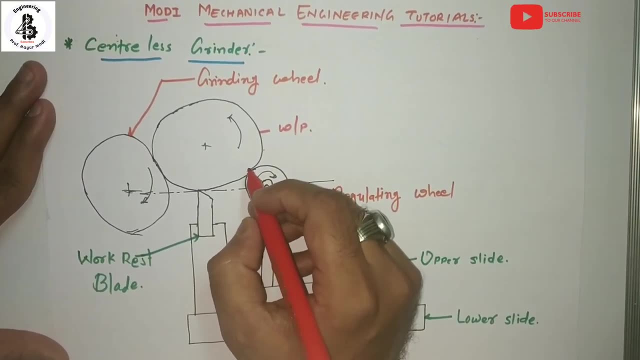 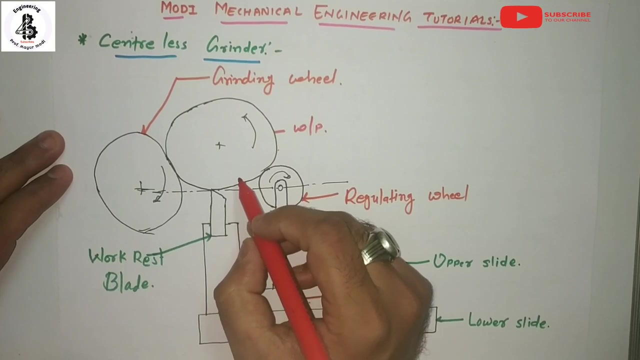 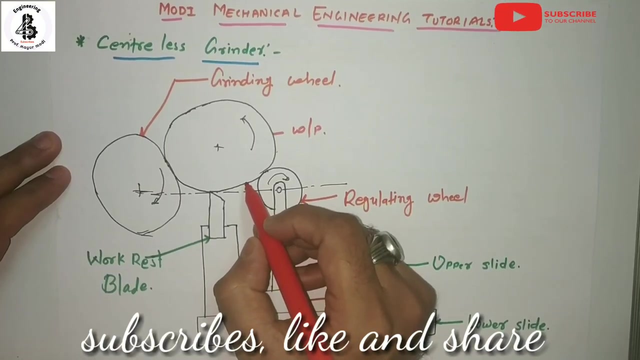 Two regulating wheel, or you can say one regulating wheel, one grinding wheel and in between that will be the workpiece, material for making the any kind of operations onto the external surface of the job. So just you can see, the workpiece is not held onto the centers but drivers and other fixtures that will be hold the workpiece and also provide the rotations. 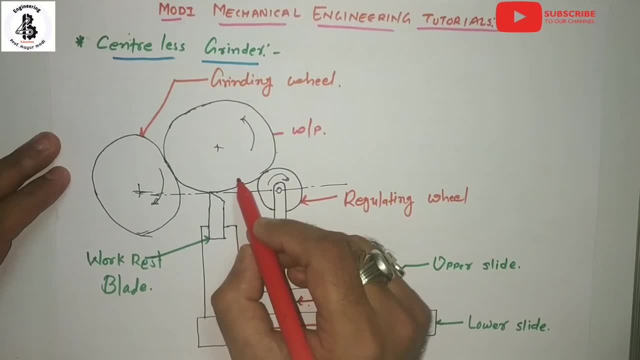 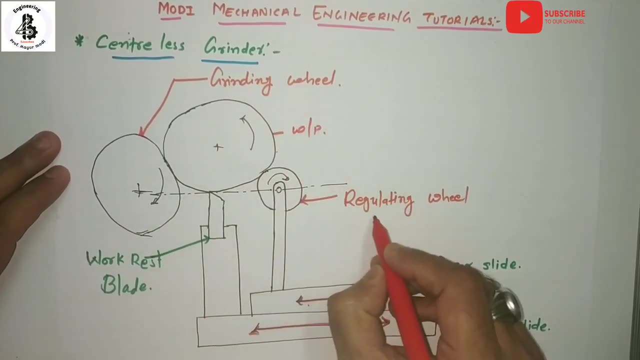 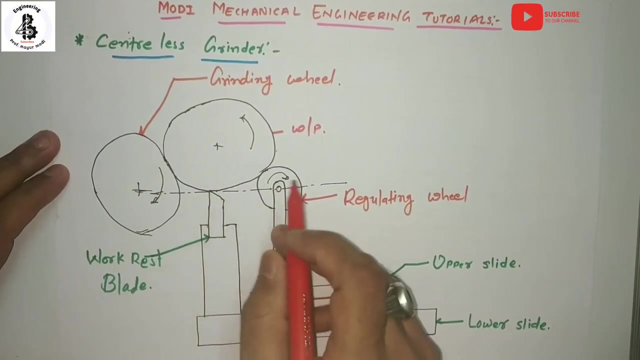 So just you can see into the diagram of the centerless grinding process. So basically centerless grinding process it will be consist of the grinding wheel, regulating wheel and the work rest. So basically workpiece that will be onto work rest and both the side, one side that will be the grinding wheel and another side that will be the regulating wheel. 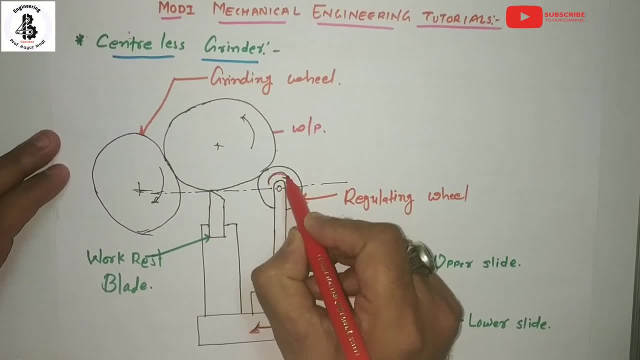 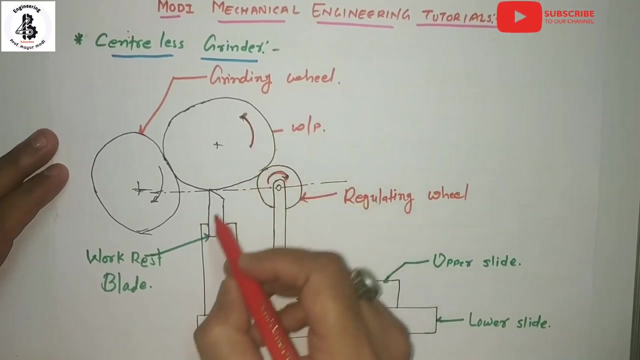 So this regulating wheel, it will be rotate into the clockwise directions. So according to that rotations, the periphery of the regulating wheel it will be attached with the Workpiece periphery so that will be rotating into anticlockwise and that will be also supported onto the work rest blade. 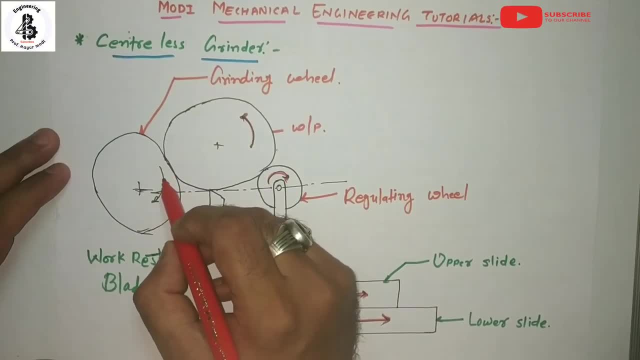 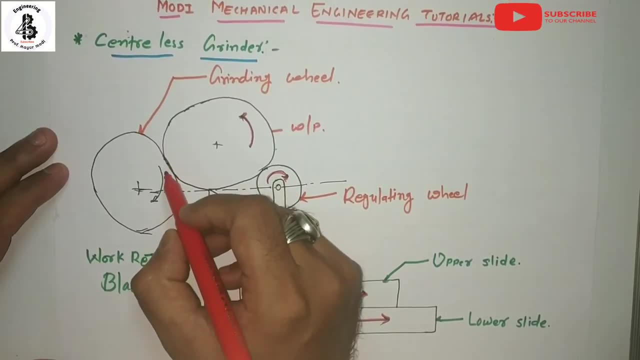 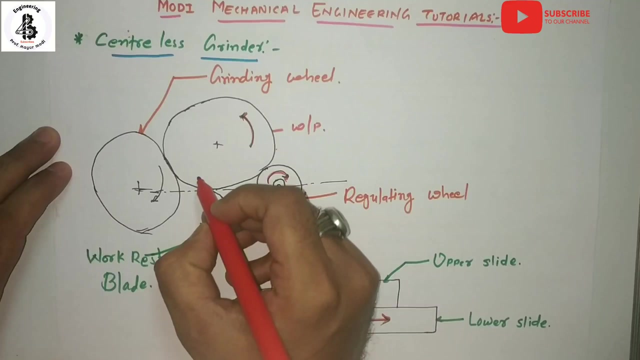 On another end that will be the grinding wheel. So basically, with the application of this grinding wheel that material removal take place in the form of the powders. So you can easily doing an external work onto the cylindrical job, taper job. or you can say: 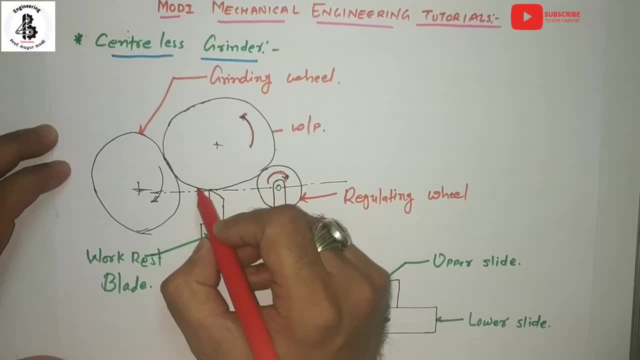 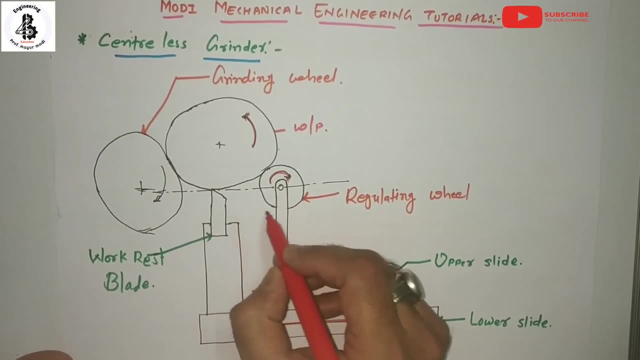 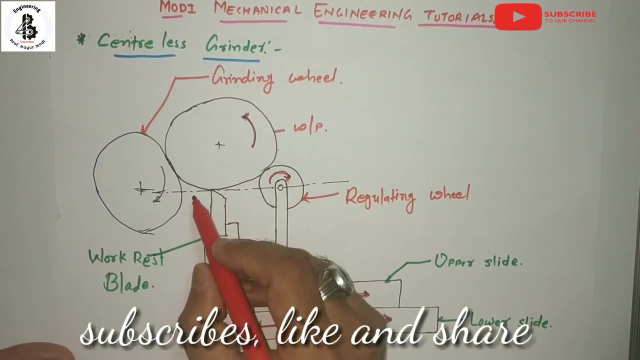 To form the new surface onto the workpiece materials. So just you can see over here the work rest is looking in between the regulating wheel and grinding wheel And just you can see the work piece that will be placed onto the the work rest. So this is our work rest blade. 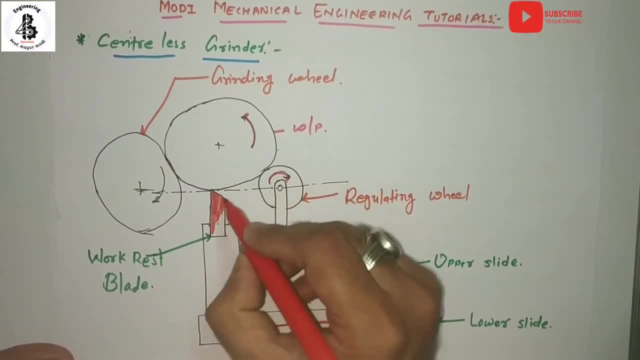 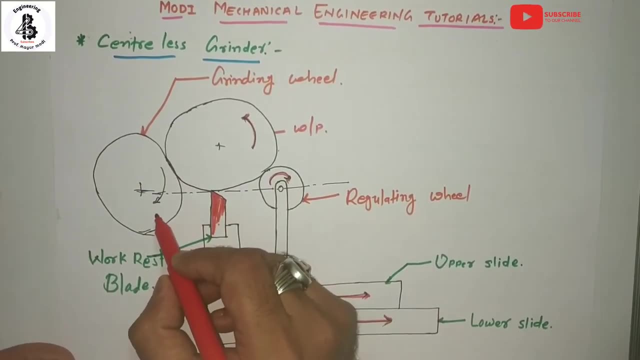 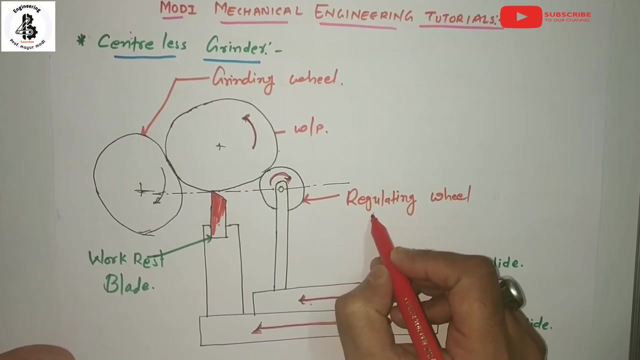 So providing support in between grinding wheel and regulating wheel. So the grinding wheel is In between the grinding wheel and regulating wheel, is mounted in the wheel head, which is rigidly fixed to the machine members. or you can say the regulating wheel, this one and the work rest blade. that will be providing the basic support. 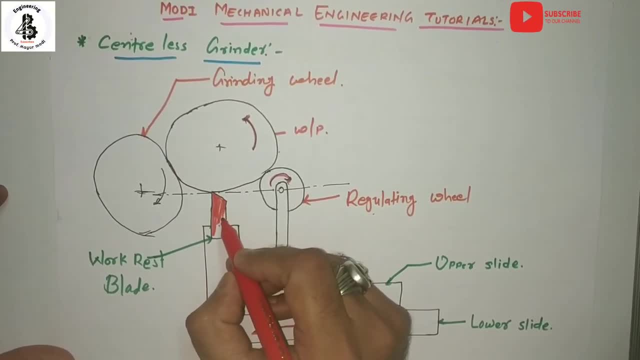 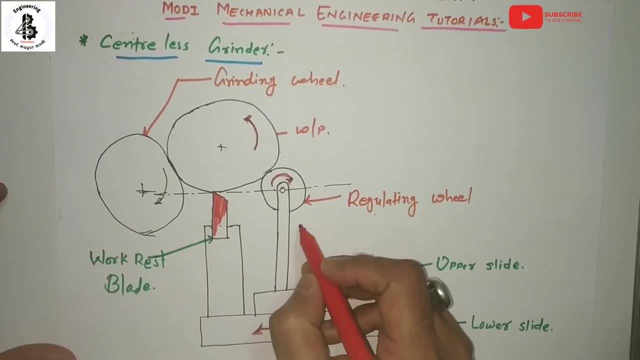 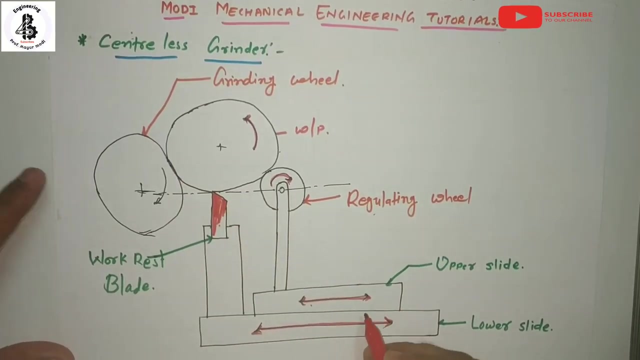 during the machining operations, or you can say grinding operations. So the regulating wheel is also controls the speed and feed of the work piece. So, whenever that will be, the dimension is permanent changing. so by the application of the lower side and upper side, this column, or you can 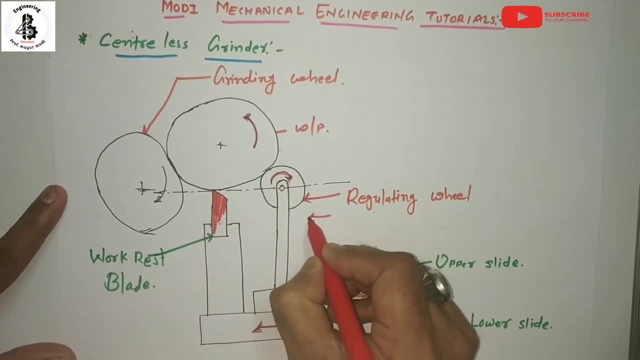 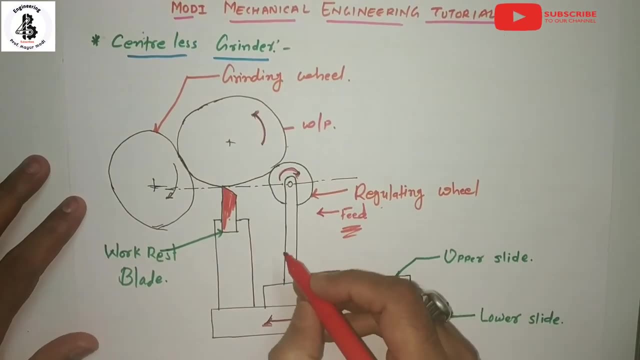 say this: supporting regulating wheel. it will be moving into this directions for providing the feed. Now, from the figure just you can see the regulating wheel is mounted on the work piece. So this is the regulating wheel which is mounted on the work piece. Now, from the figure, just you can see the regulating wheel is mounted on the work piece. So this is the. 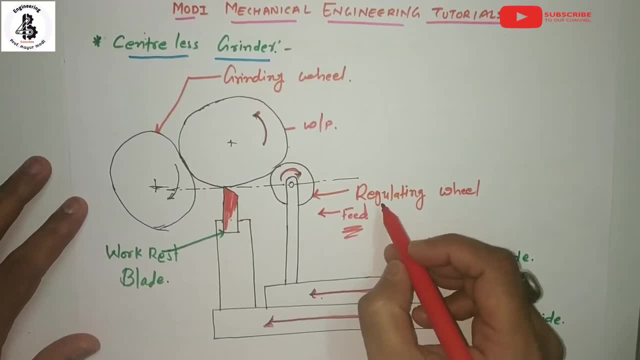 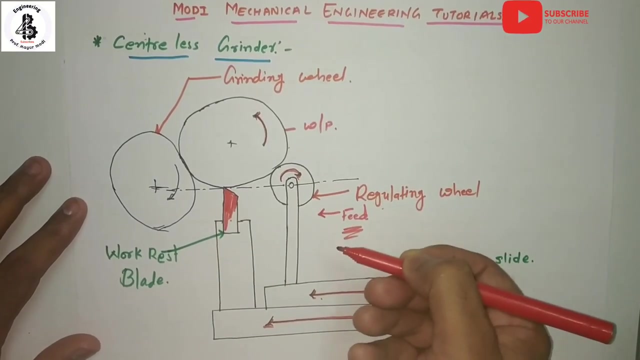 on a side so that that will be its axis of rotation, can be moved towards, or you can say away from the work rest, So that will be rotated into clockwise direction, so that will be away side, so that will be need to be controlling this distance by the application of the feed and this. 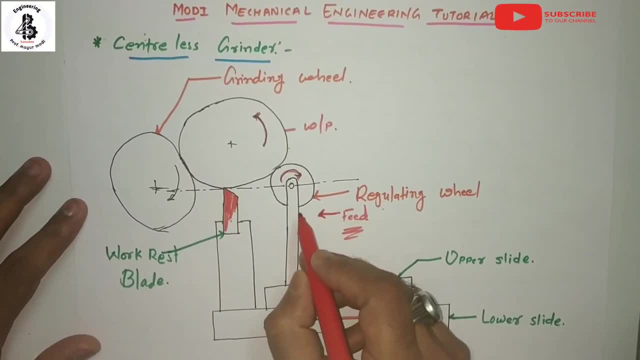 adjustment is required to accommodate the jobs of the different size, of the diameters of the machines to be grind. So the work rest have also adjust in a vertical directions as per the requirements of the different shape and size of the jobs. So in case of the centerless grinding process, if the 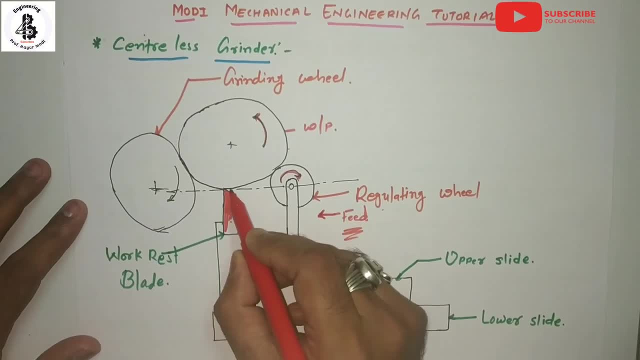 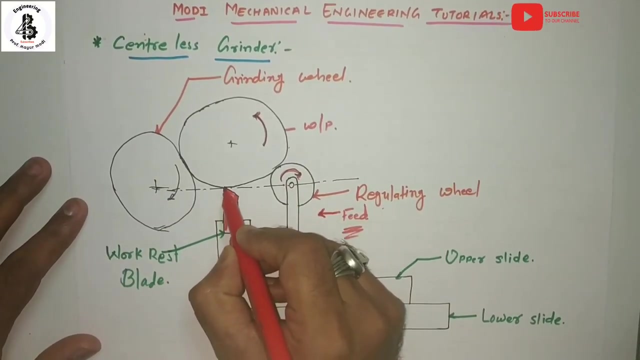 axis of the job is too near to the center line. So this one that will be the center line of the wheels of the job, is well supported but not suited for the proper grinding. So that will be the center line that will be the supporting rate point. So basically, this periphery. 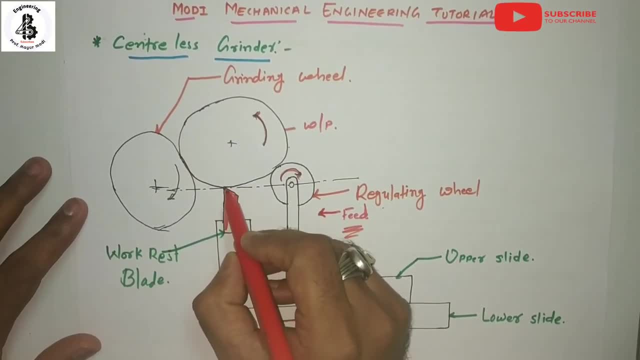 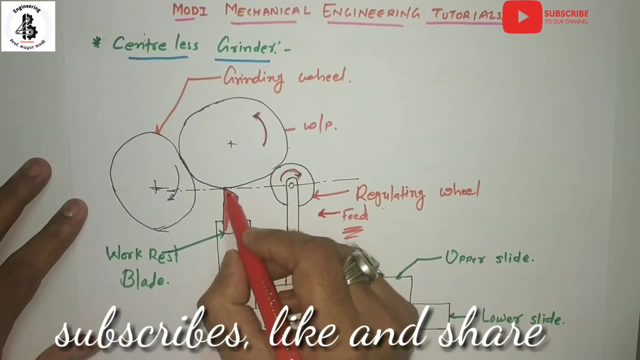 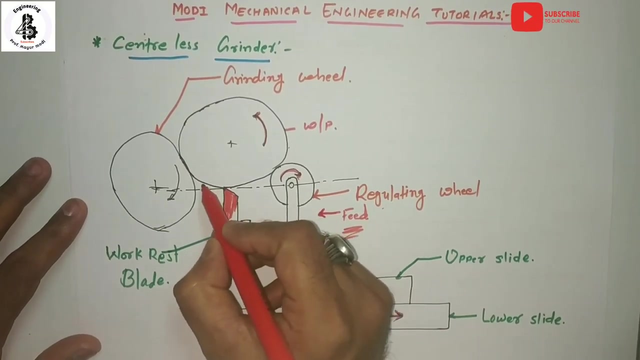 will be passing through these lines. So that would be having a good grinding efficiency. Also, if the job axis is too far above the plane containing the axis of the grinding and regulating wheels, the job is not properly supported. So during that it will be not over here, it will be just it will be far. 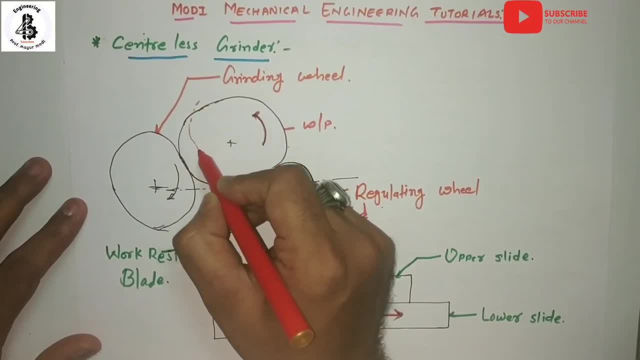 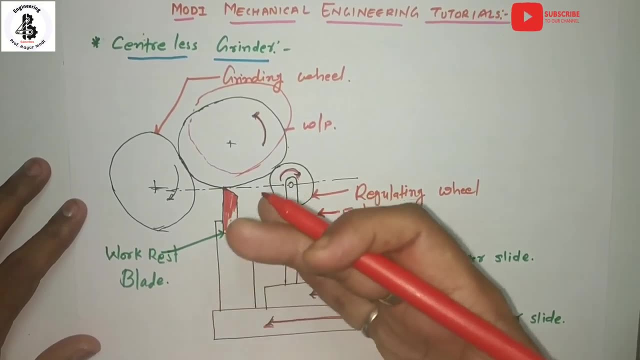 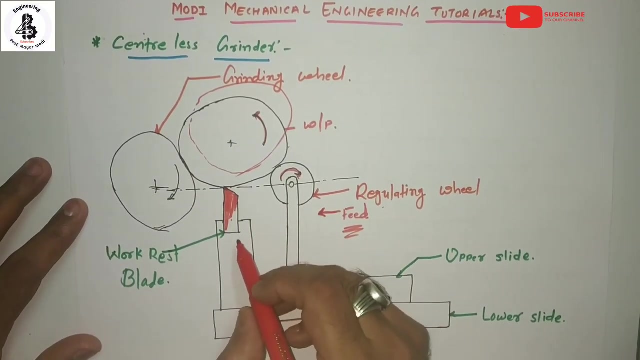 from this point. So like this- suppose this one is my job. So during the centerless grinding process that will be increasing the vibrations during the centerless grinding process. So usually the height of the job center line from the center line of the wheels it will be kept half of the diameter of the job, with the maximum of the 12 mm. 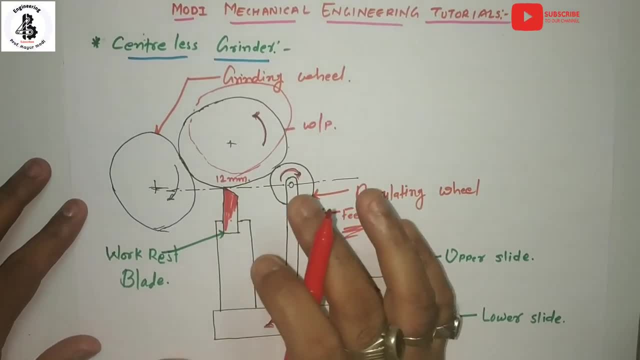 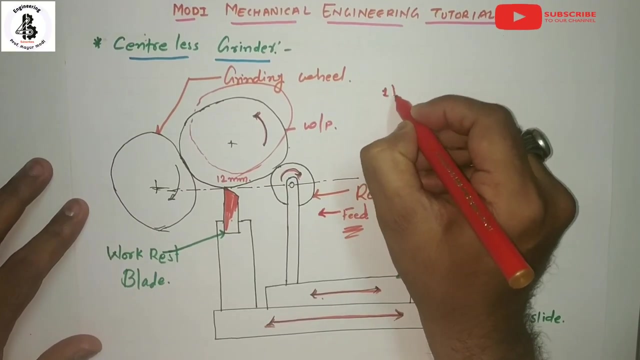 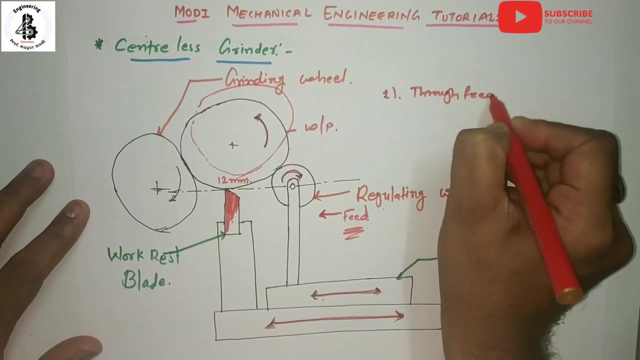 or you can say up to 12 mm, So you can performing satisfactorily, or by the centerless grinder process. So basically, the centerless grinding can be done by the differing methods. So first one, I think it will be the through feed centerless grinding. 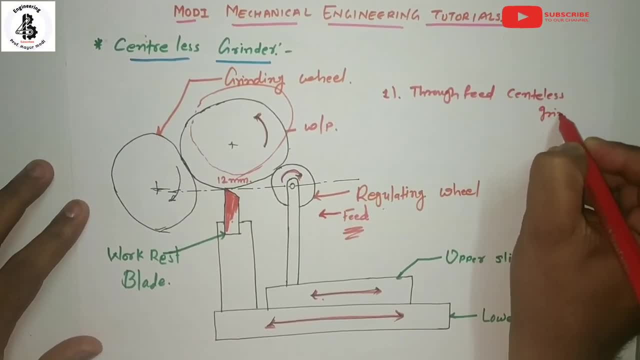 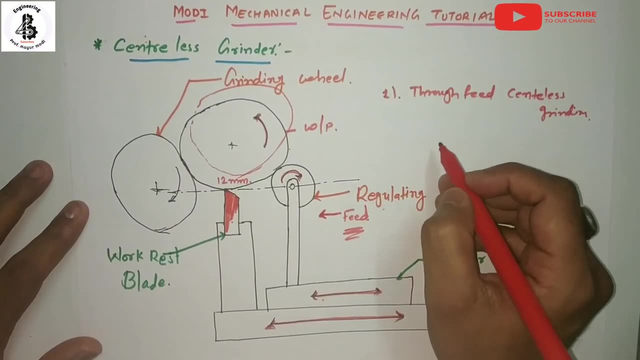 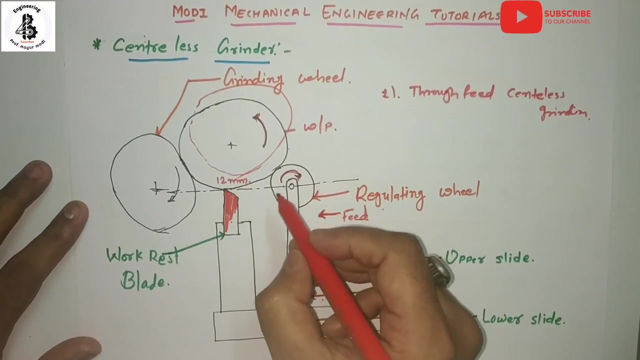 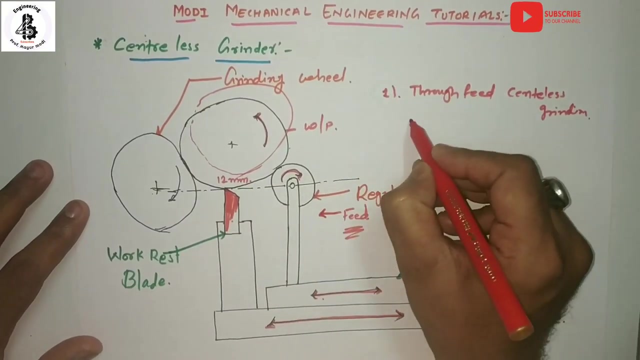 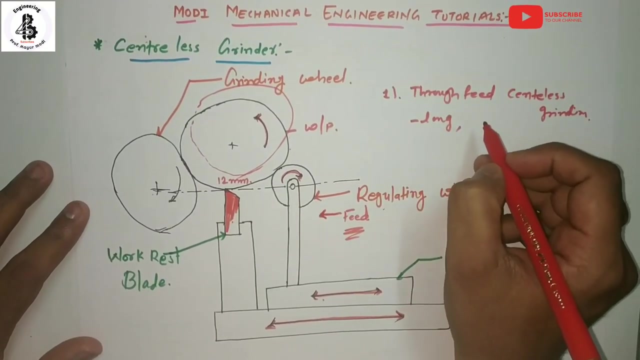 so in case of the through feed centerless grinding speed through feed centerless grinding process, the work material that will be completely through the pass between grinding wheel and regulating wheel, So it is useful for grinding of long shaft, slender shaft, without the shoulders So you can performing the centerless grinding. 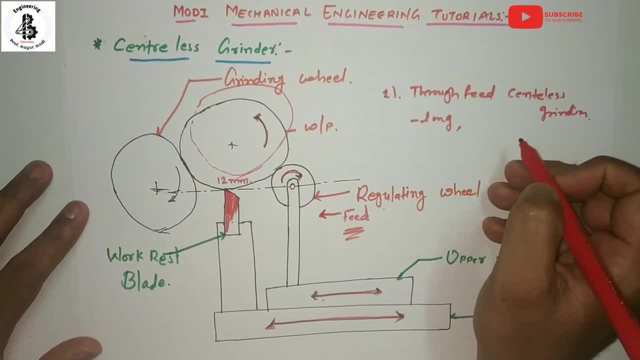 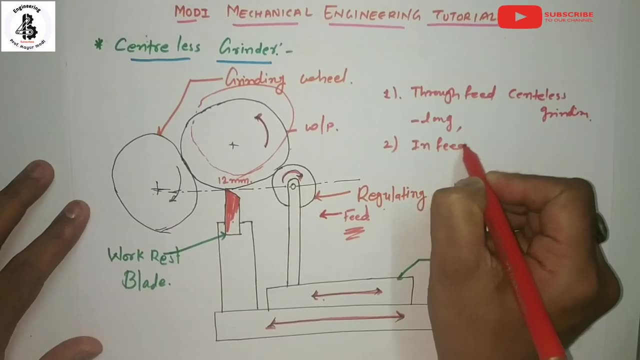 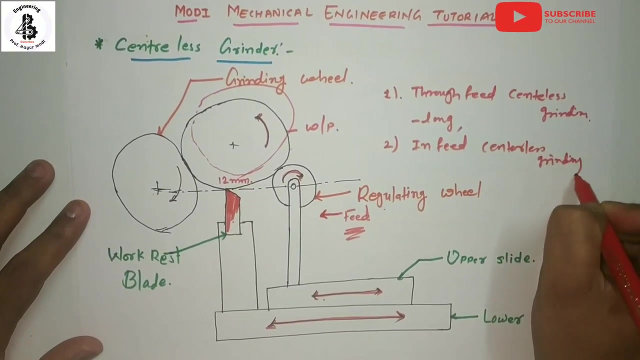 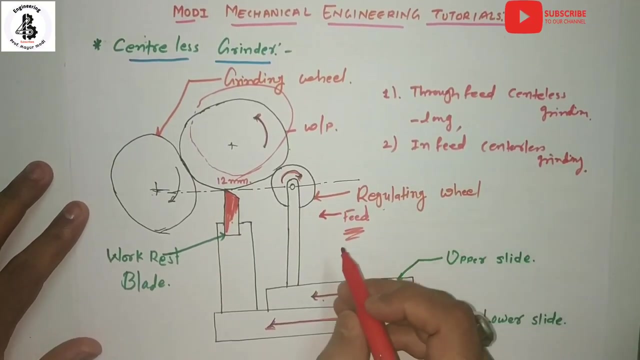 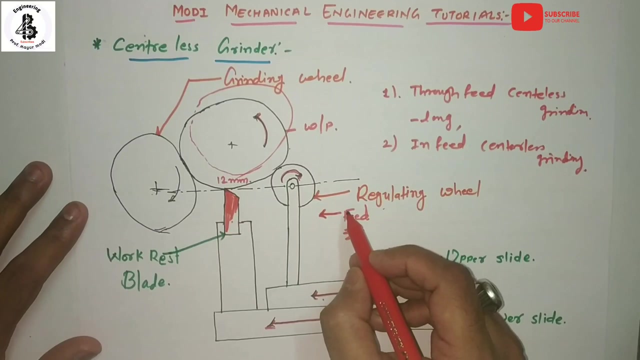 operations with the through feed centerless grinding methods. second one that will be in feed in feed centerless grinding process. So in case of the in feed centerless grinding process, basically suitable for axis symmetrical jobs. So this grinding is similar to the plunge grinding or you can say form grinding processes. here the regulating wheel is drawn back. 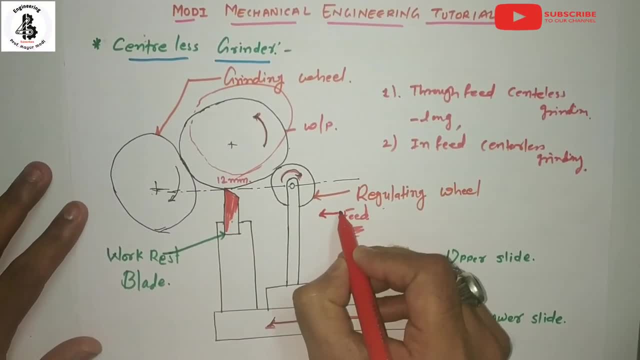 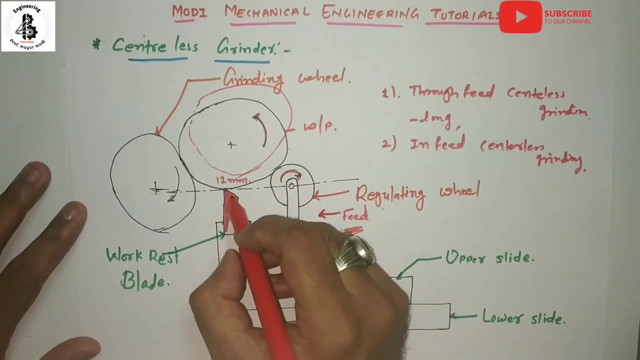 so that will be into this directions, so that the job may be placed onto the rest blade and then it is moved onto the feet, the work against the grinding wheel. so that will be only touching with the grinding wheels, so that will be disengaging during the in-feet centerless. 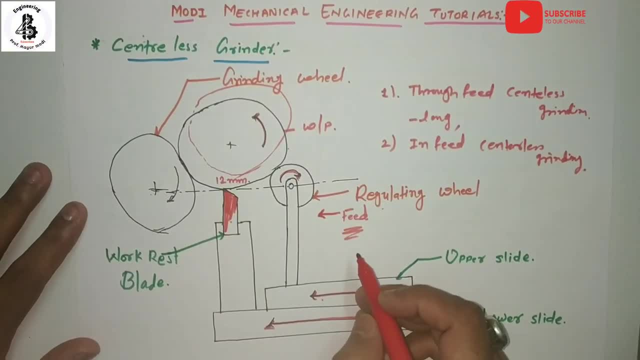 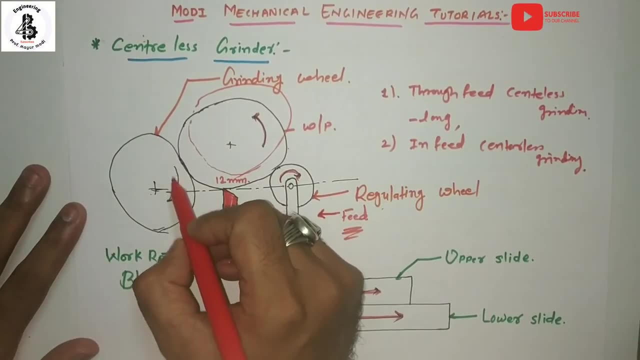 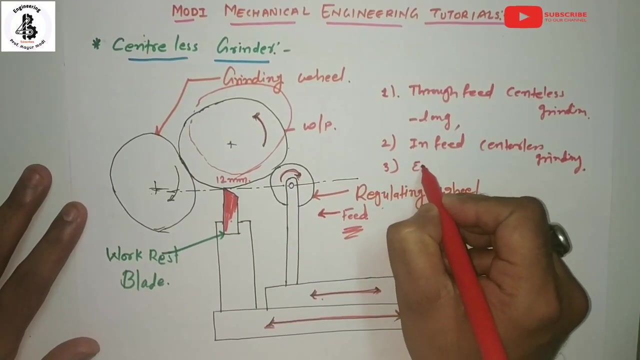 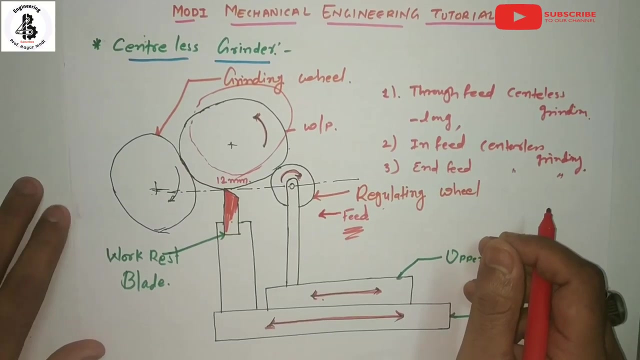 grinding process. so the end stop is kept to prevent the step jobs from the moving beyond the limits, so you can performing with the only help of the grinding wheel. and the third one, so end feet, centerless grinding process. so in case of the end feet grinding which is suitable for the 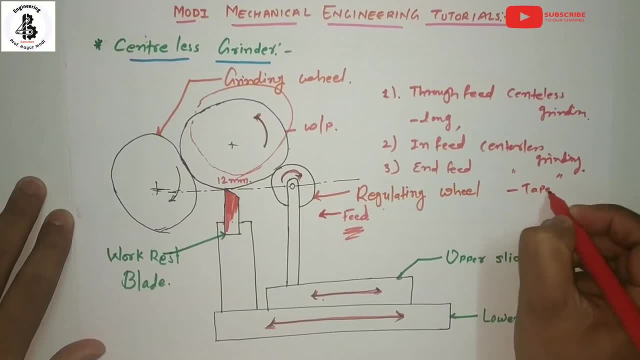 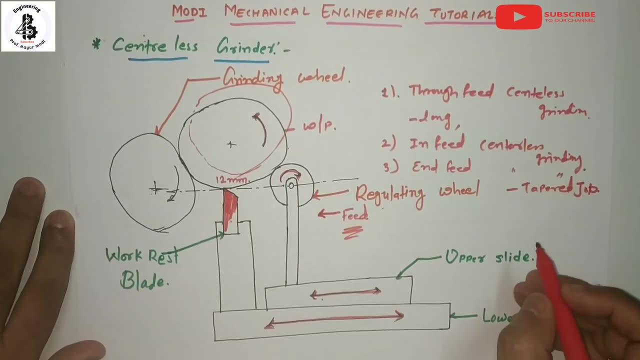 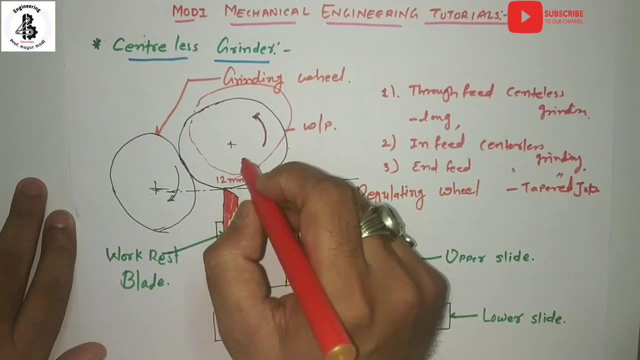 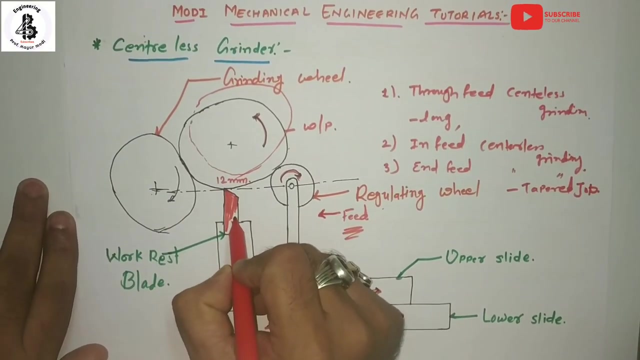 tapered job and basically to make the form tapered onto the work piece material. so work piece is fed lengthwise between the wheels and that is ground as the advance until it reaches the end stop. so the regulating wheel and that work rest are not withdrawing the work piece material. so the 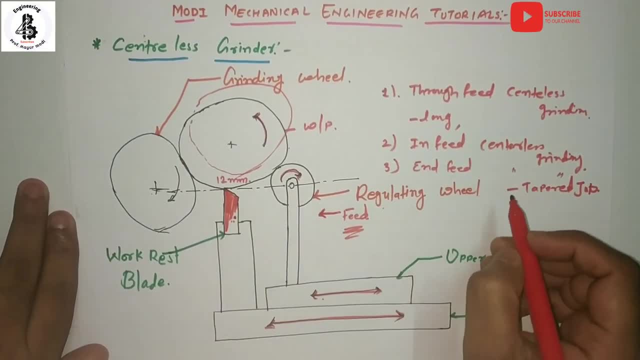 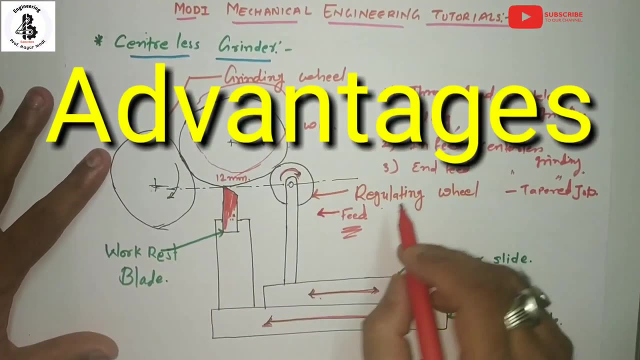 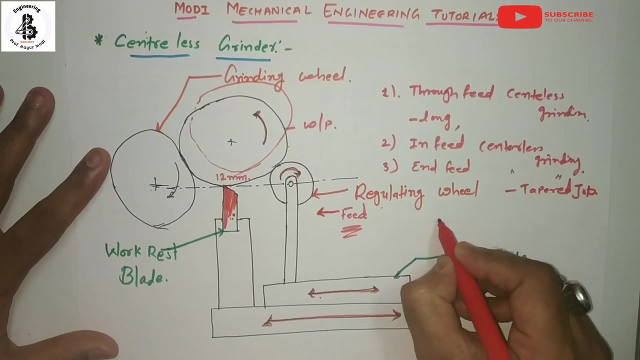 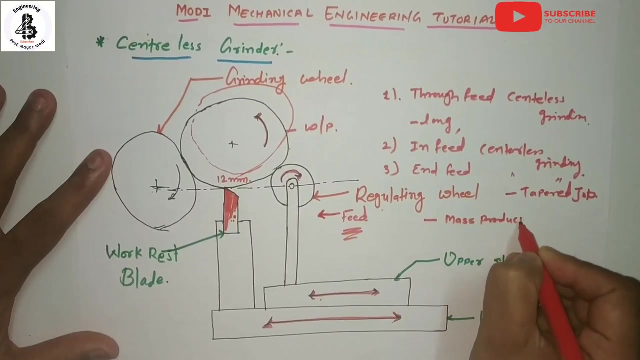 in this case of the and feet centerless grinding process. now some of the advantages discussing for centerless grinder process, and that will be this process is a continuous process and useful for the mass productions. so here i would like to write down for mass production: second one, as a true floating condition: 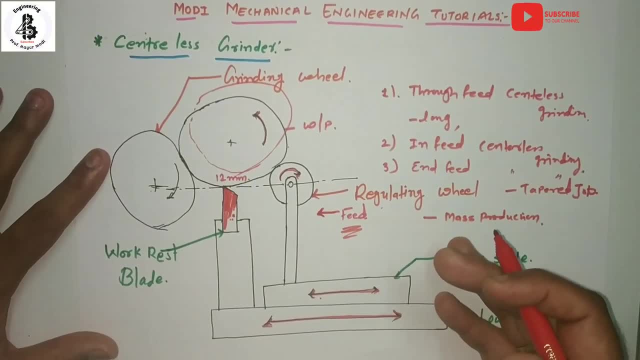 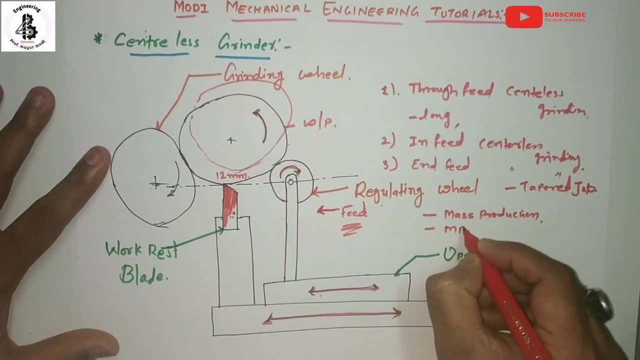 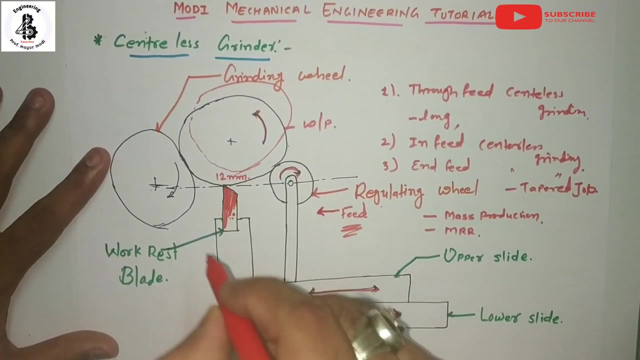 during the grinding process, the material required to remove is very less so during this process. the emar, that will be the less material removal rate. one more, and that will be the work piece being supported, true, its entire length, suppose this one is considerably the one kind of cylindrical, and that will 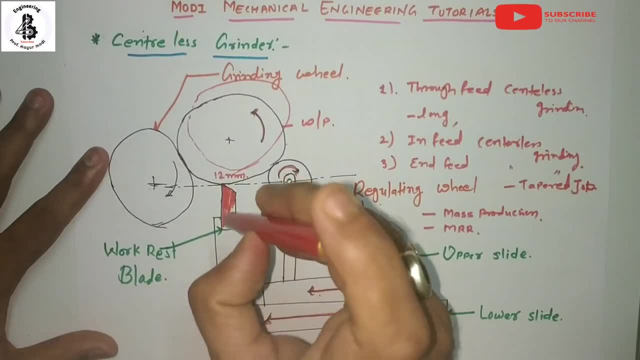 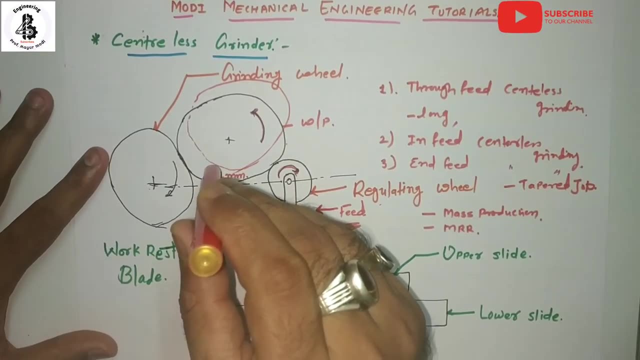 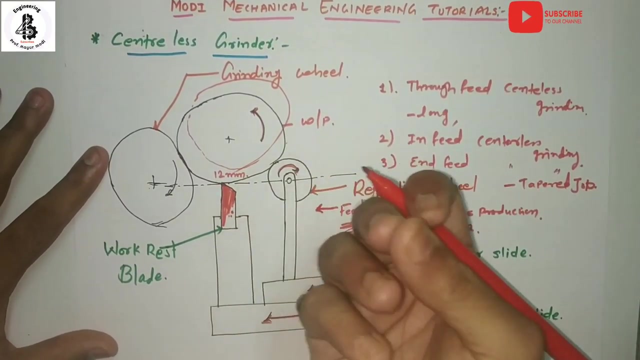 be supported by this works wrist blade throughout the land. so no deflections, or Or you can say no chatter, stick place Right. And one more thing: the slender work piece- or you can say small size, or you can say fragile jobs- can be ground easily. 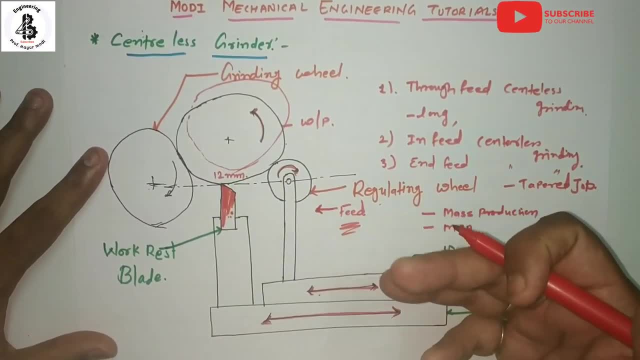 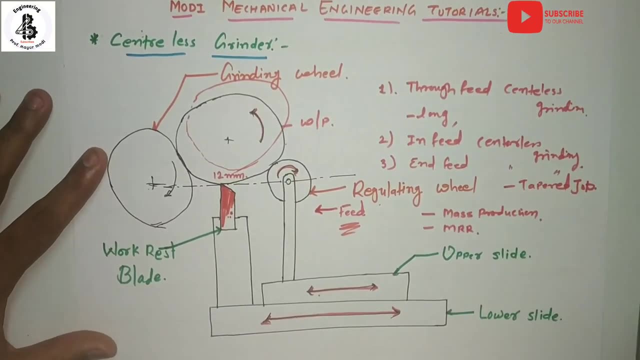 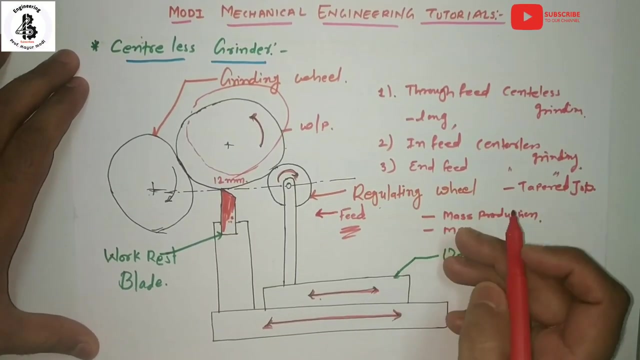 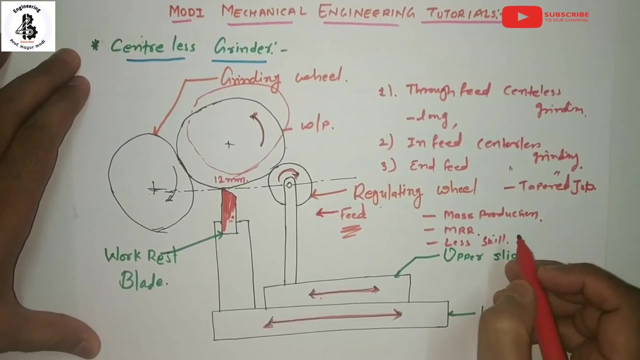 So you can performing the centerless grinding process without any kind of difficulties And that would be also increasing the accuracy as well as the good productivity into the productions. Size and specification control is good for the centerless grinding process, Less skill of the operator. that will be also good things for increasing the productivity as well as the accuracy. 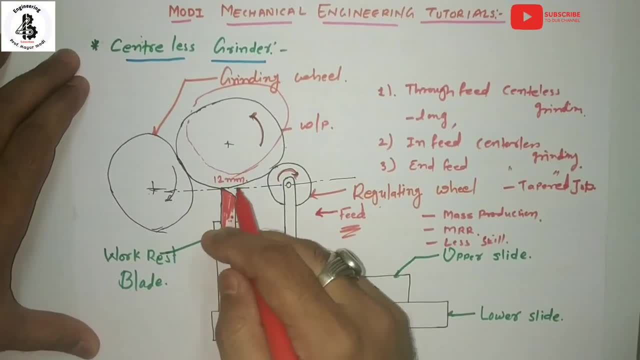 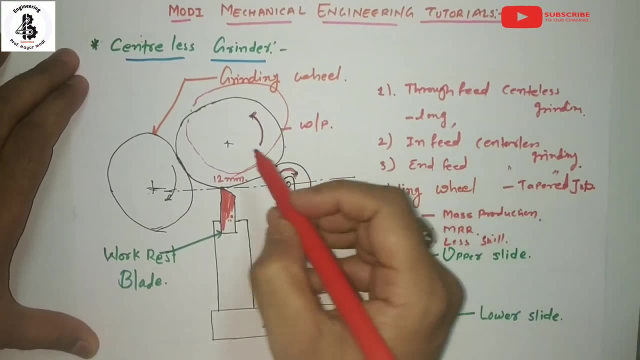 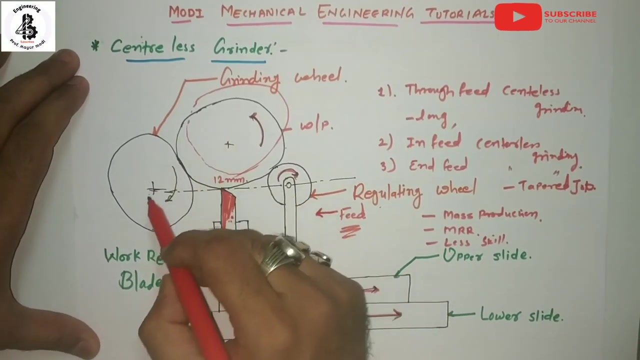 No center holes, or you can say no chucking, or you can say mountings of the job onto the mandrel, or you can say other holding devices are required So that components, or you can say work piece only supported onto the work rest blade. And from another two side, from one is the gunnery- 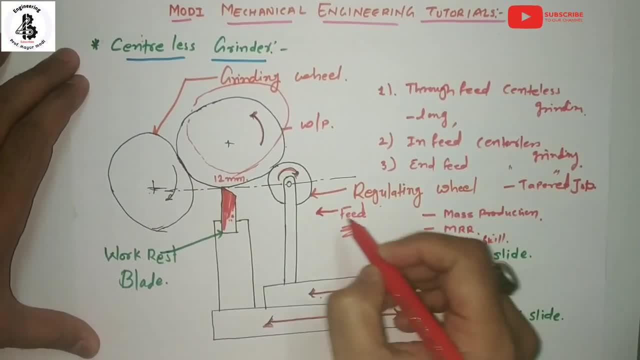 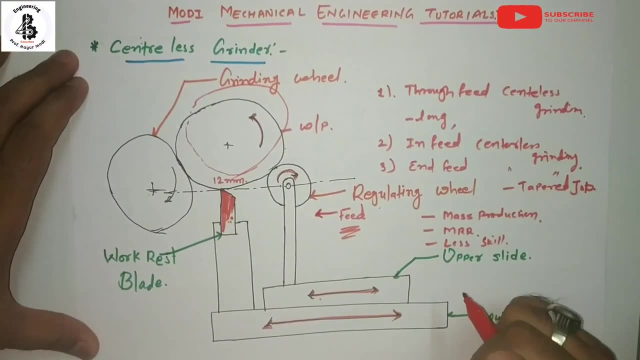 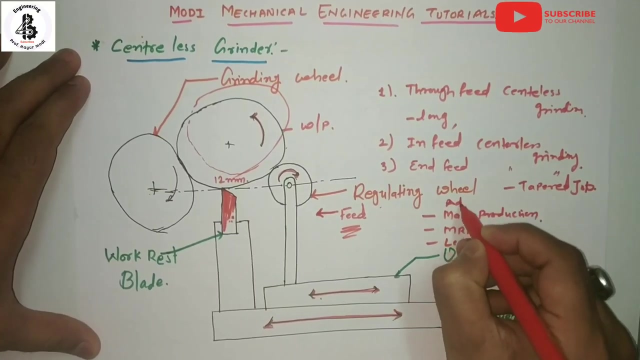 One is the grinding wheel and another that will be considering as a regulating wheel. So that will be supported in between these two Right. So there is no additional support required for the centerless grinding process. So these all are regarding to the advantages of the centerless grinder process. 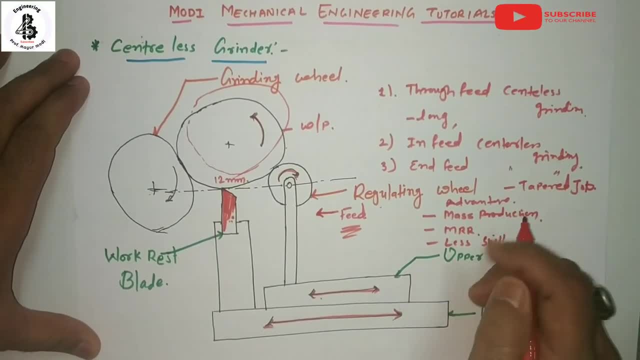 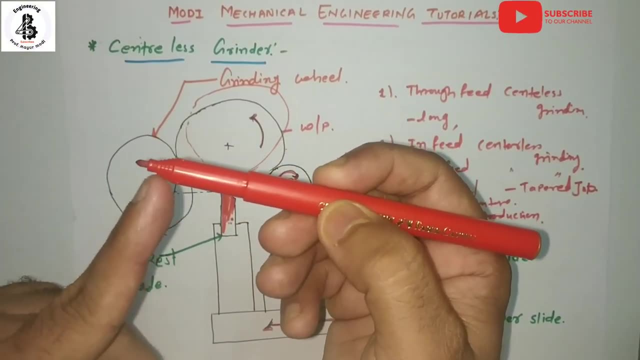 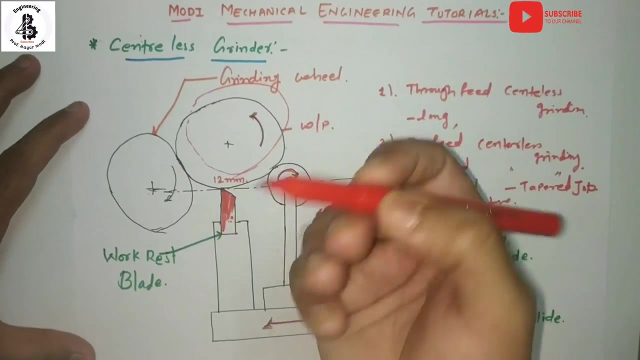 Now, every process that will be having some limitations and that will be the work piece having a multiple diameters, So such kind of tapered section that you can find over here, Right? So such kind of job that will be difficult to handle into the centerless grinding process. 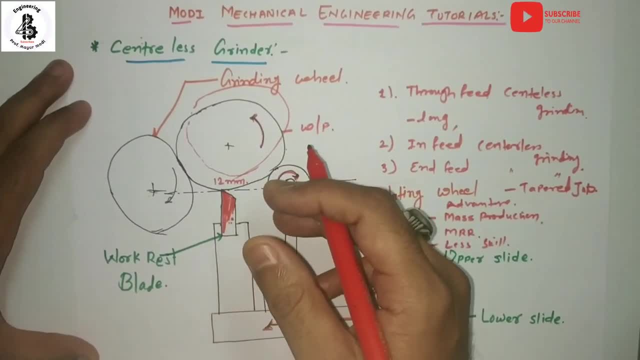 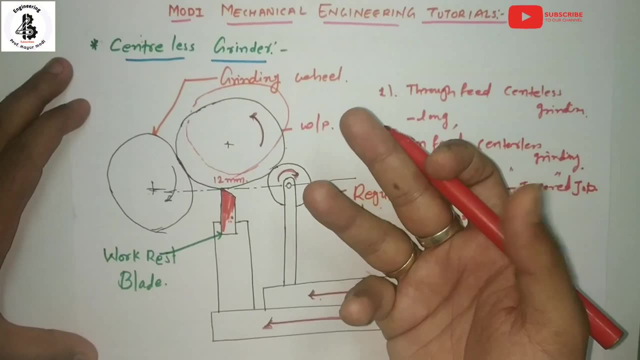 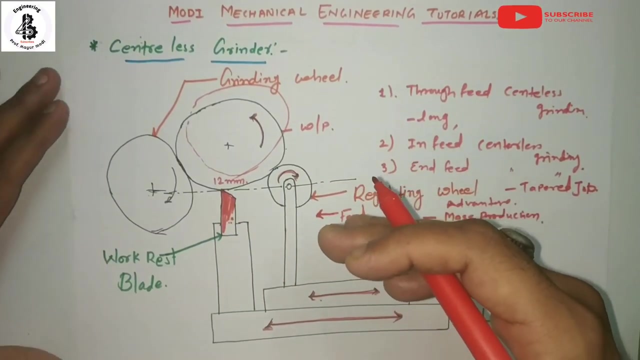 And for hollow work piece there is no any certainty that are the outside diameter will be the concentric with the inside diameters. So if that will be the different kind of thickness of the cylindrical job, So that will be the control of, So that centerless grinding process that will be having a difficulties.